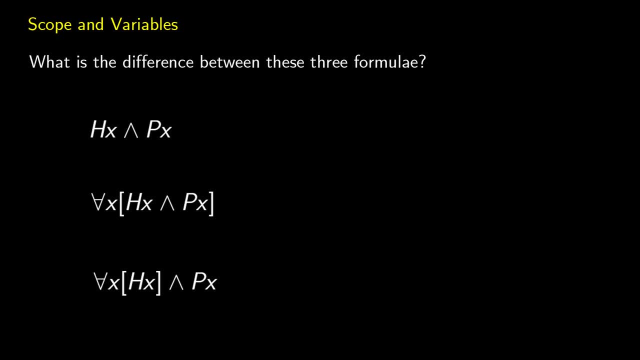 Before we can do any sort of translation in predicate logic or do proofs, we need to understand what scope and variables are. So, to introduce this, I want you to take a look at these three formulas and think about the differences. Well, the main difference in each of these: these both have hx and px, but it's this quantifier for all x. 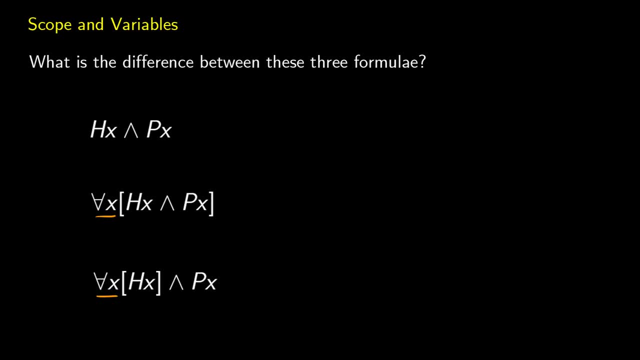 In the first one there is no quantifier, so it's just hx and px. In the second one, there is for all x, and hx and px are in these brackets, which basically means that the for all is talking about both h and p. 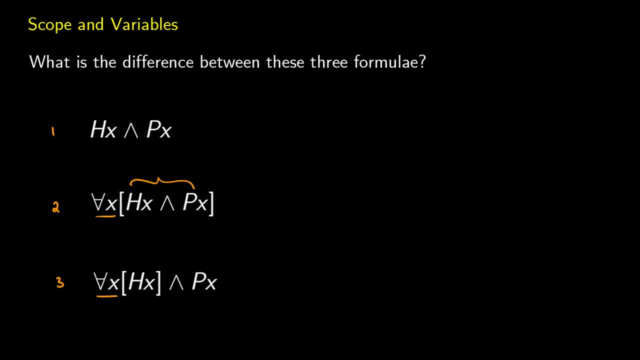 And then in the third one, we have for all x, hx in brackets, but then px is outside of the brackets. Now, each of these three different formula have different interpretations, and we'll have to talk about scope and variables in order to understand that. 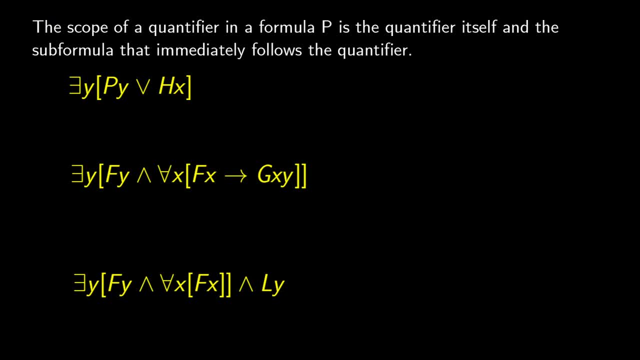 So let's start by talking about scope. And here is the nice point. This is a formal definition where we say: the scope of a quantifier in some formula is the quantifier itself and the subformula that immediately follows the quantifier. So in terms of regular English, what this means is, if we say: focus on the scope of exists a y in this first formula, 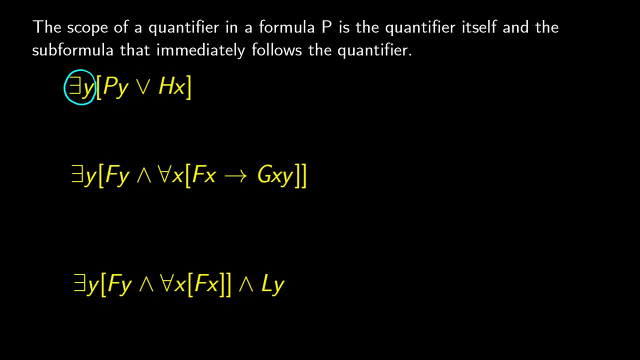 The scope of exists. a y includes itself and everything following it in brackets. So I like to use square brackets to show scope Because it's easier for me to keep track of, But of course you may see something in a textbook that looks a little bit more like this. 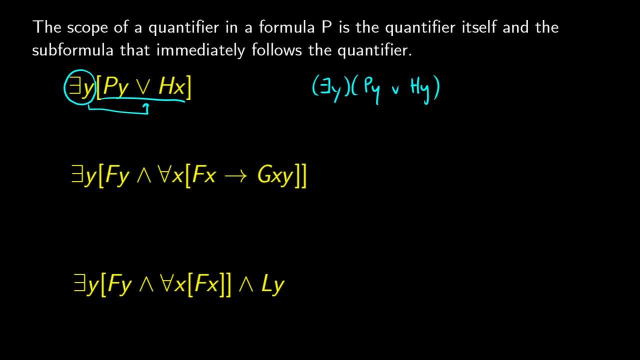 py or hy, And these all use the regular parentheses. This is the same thing. So we just take the quantifier itself and everything in the following set of brackets. We need to make sure that we follow the left bracket and we find its corresponding rightmost bracket. 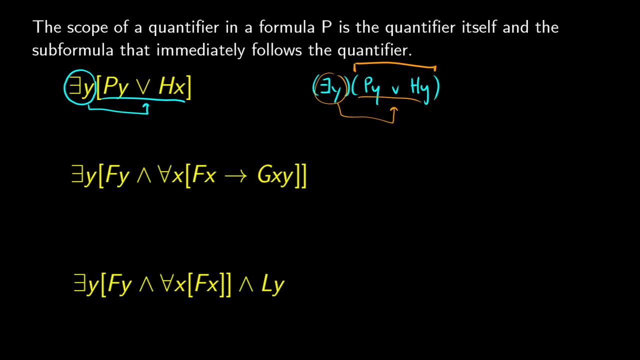 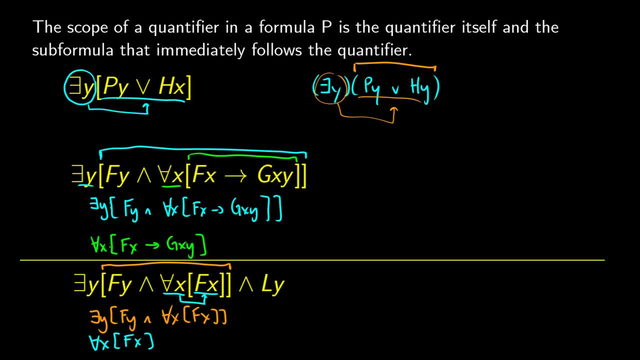 So those are our three questions there that can help us identify the scope of quantifiers. Now, this is just step one. Step two is taking a look at the variables inside of these predicates, like p, y and h, x. so looking at the y and x there and determining what type of variable they. 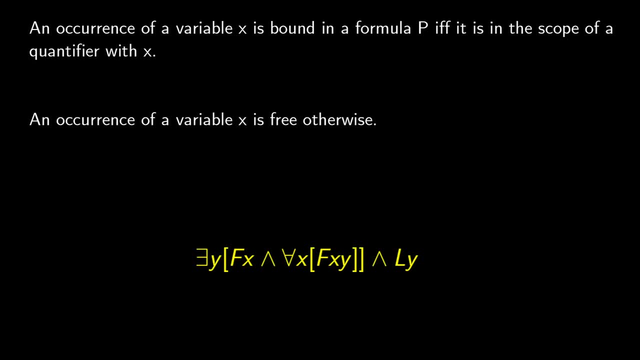 are. So if, and let's just illustrate this, so I'll write out a little formula. first let's just do something really simple, like for all x, fx, An occurrence of a variable x is bound in a formula if it's in the scope of a quantifier with x. So in other words, if we see x as a. 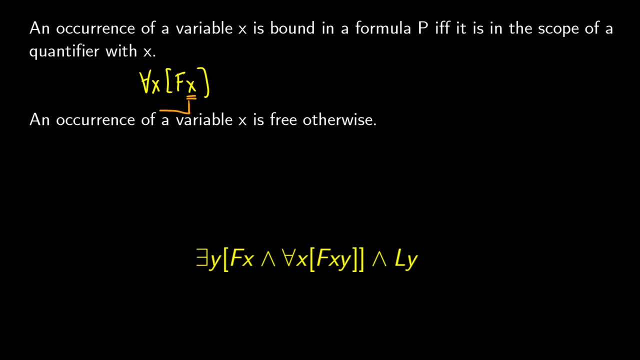 variable. here we need to say: we need to see if it's in the scope of a quantifier with the same variable. If so, then we need to see if it's in the scope of a quantifier with the same variable. If so, then this one instance of the variable is bound. But we could have multiple variables. 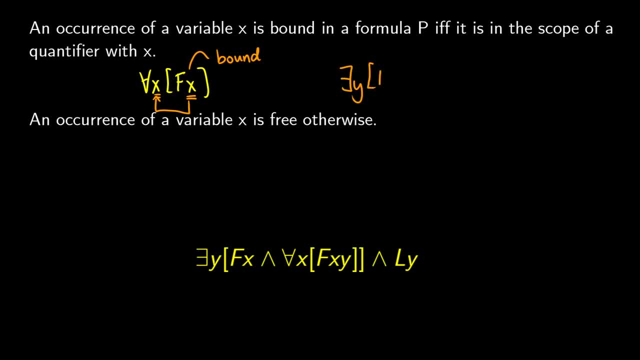 so let's say we have something like exists a y and then we have p y y. Then we would say that, okay, each of these ones are bound. so it's not just an entire formula that's free or bound, it is each individual variable. So the first y in p y y is bound, as well as the second y in this. 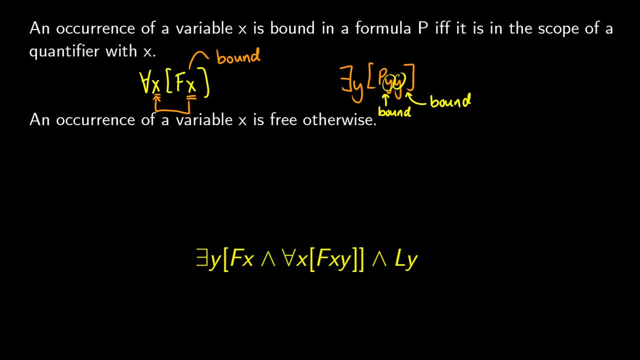 case. Now, if it's not in the scope of a quantifier with the same variable, we say it's free. So, for example, if I have for all x and I use fy instead, I need to take a look at this y here And what I'm. 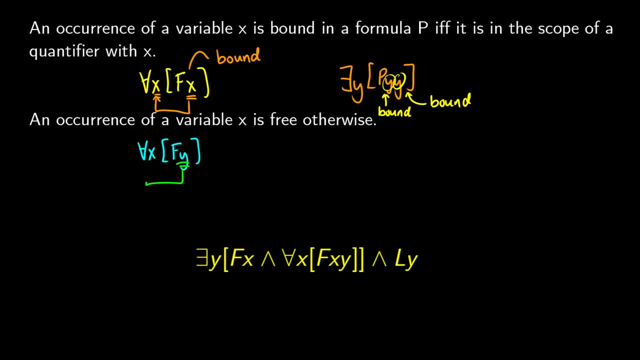 looking for is a quantifier with another y in it where that fy is in its scope. But we don't see one. So because there's no y quantifier that is scoping over, we don't see one, So we don't see. 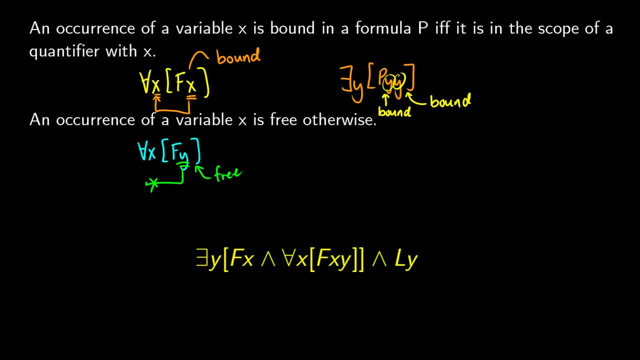 another fy. here We say: this is a free variable. So how could we make this a bound variable? Well, one way of making this a bound variable, of course, is just to change this for all x to all y, and now suddenly this would be bound. But that's not what we had in our original question. 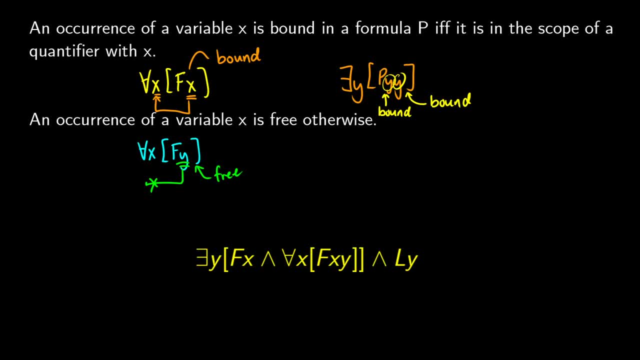 we just had for all x, fy. So let's do an example with this formula below, So you'll recognize this from the previous slide. So we just changed one little thing around here. So we have exists a y, fx and for all x, fxy, and. 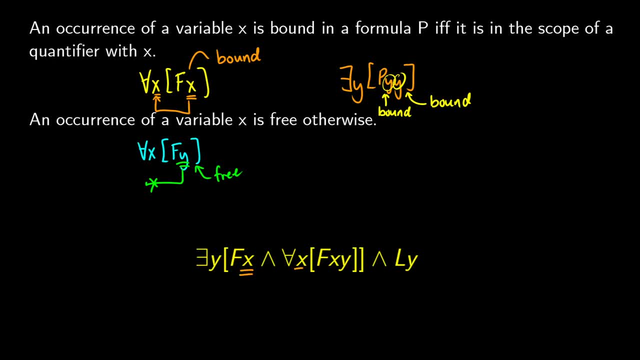 ly. So basically for each of these variables, so fx and then fxy, so xy there and y at the end, and ly, we have to state whether it's free or bound. So for fx, we're looking for an x quantifier. 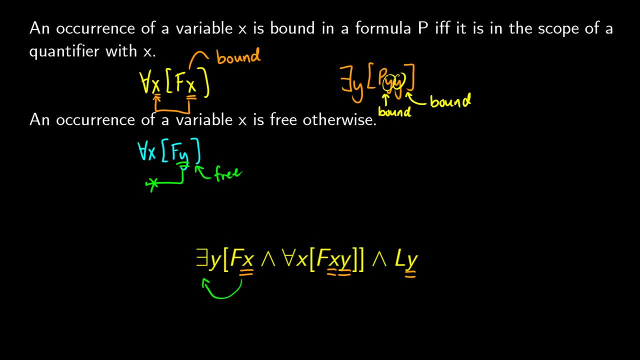 somewhere to its left, outside of the brackets. We don't find one. Therefore, this x in fx is free, But in fxy we do find an x quantifier, right outside of its brackets. We have for all x, fxy. So this one is bound, this x. Now what about the y? 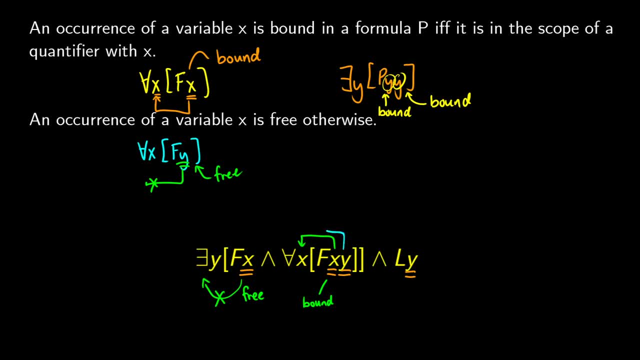 Well, although we don't find a y quantifier immediately outside the brackets, it's still in the scope of a y quantifier. So the existential y at the front of the brackets is bound. So we don't have a bound at the front that is in the scope or it scopes over fxy. So this y is also a bound. 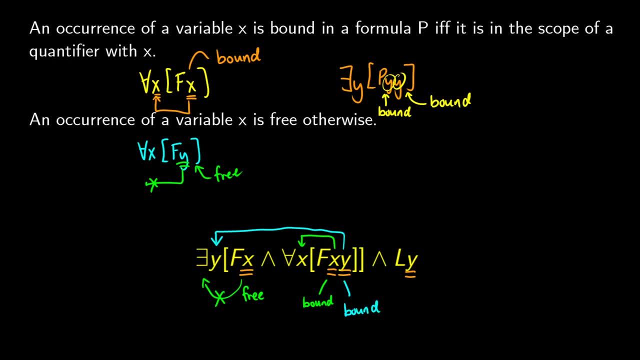 variable. But what about this last one? So ly? Well, it's not in any brackets, There's nothing scoping over ly here, So there's no y quantifier that connects with it. So this case of y is free. If we wanted to make this bound, we would have to do something like and for all. 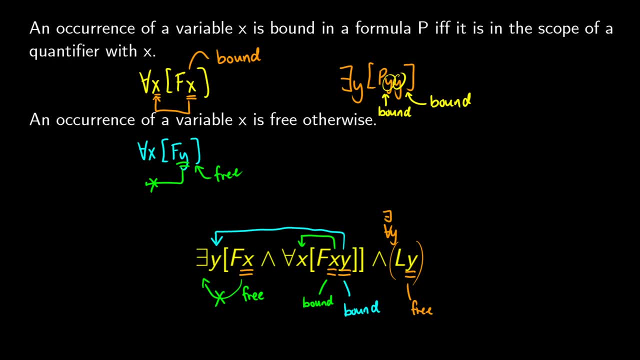 there exists a y ly or there exists a y ly, But we do not have that. This ly is out of the scope of the other two quantifiers. So that's a nice little formula with two free variables and two bound variables. So this is sort of step two. You understand scope and now you understand. 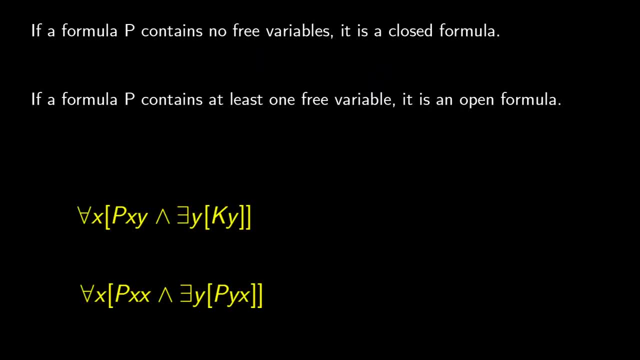 variables, And we're going to get to practice this when we talk about open and closed formula. So if a formula has no formula, then it's a bound. So if a formula has no formula, then it's a bound, And if there are no free variables, we say it's closed. Like, for instance, all x, hx is a closed formula. 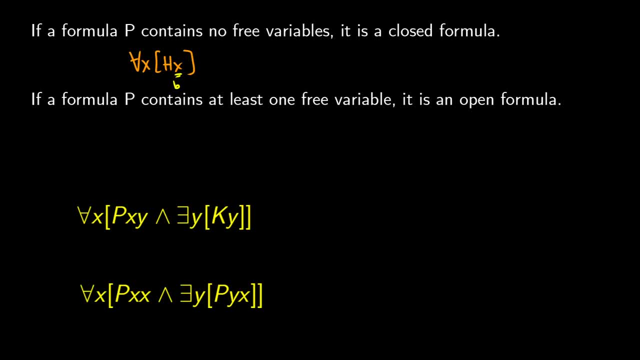 because there's no free variables. This is a bound variable. Or we could have: exists an x px and for all, y ly. This would also be a closed formula, because each of the variables here is bound by some quantifier. What this means is that it can be. 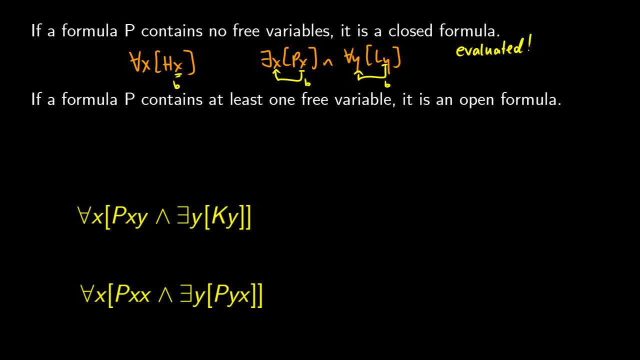 evaluated, it can get a truth value, and we'll talk about how to figure that out in a later video. but if a formula has at least one free variable, so let's say for all x, p, x, y, so in this case, sure, x is bound, but y here is a free variable, then we say this is an open formula. 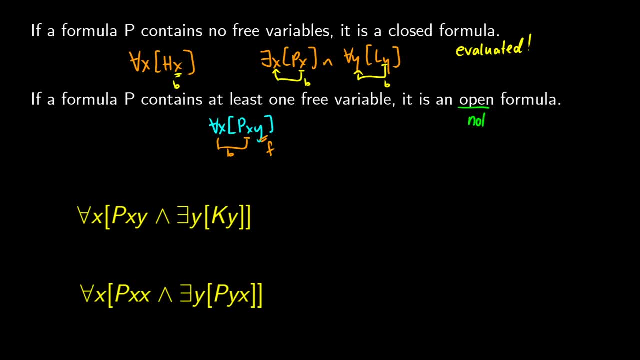 and typically this can not be evaluated, so no evaluation. this is sort of like saying something like: let's say, in math you had three plus x. well, we can't really evaluate this formula. well, a closed formula would be something more like saying three plus two. this does have an 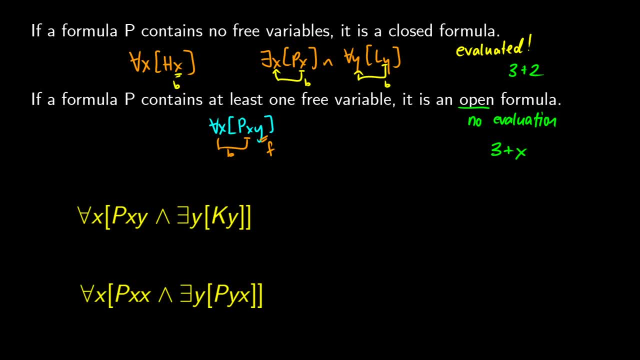 evaluation. so just sort of a little analogy, if that helps. so for these two formulas here, let's think about whether or not these are open formula or closed formula. okay, so basically, if i want to say something is open, i just have to find one free variable, and if i don't find any free variables it's closed. so in the first example, uh, basically, 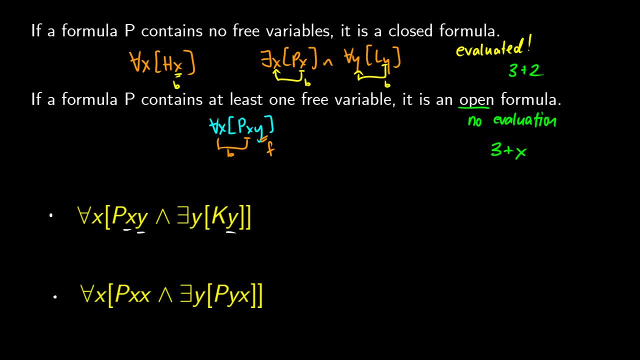 we're taking a look at all of these, so x, y and y. so the x in p x y is bound because we have that quantifier out there. but this y right here, p x y, this one is free. why? because we don't have any sort of 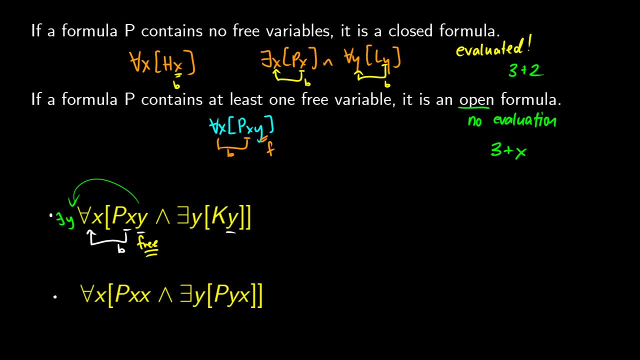 quantifier out here that has a y in it, so we don't have, say, exists a y out front. and because we found at least one free variable, we know this is now an open formula so we cannot evaluate it as is. we cannot say whether this is true or false. but in the second example here, 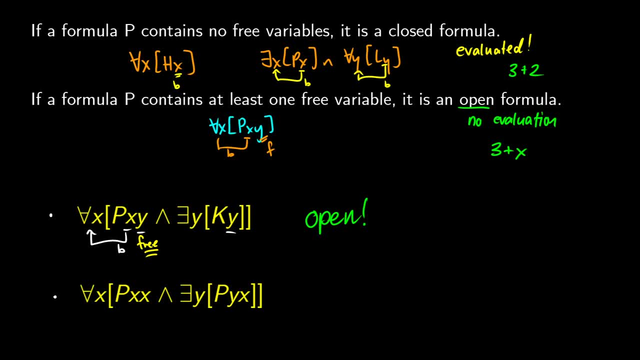 for all x, p x x. and exists a y, p, y x. well, we just have to take a look at each of these variables. so both of these x's here are going to be bound by for all x out front. okay, so that's good. uh, and exists a y, p y x. well, the y is nicely bound by the existential y there. 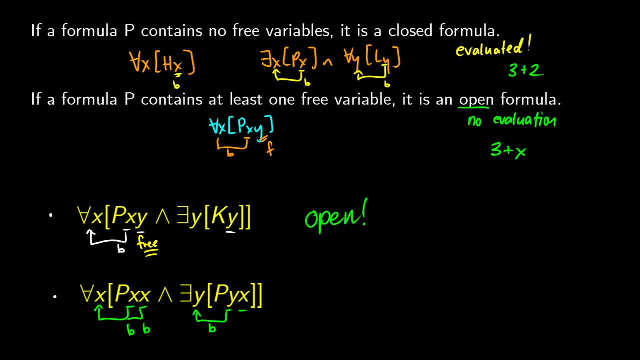 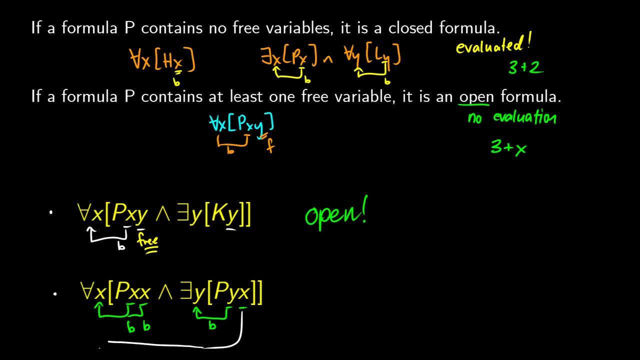 and for the x. well, we still keep taking a look at the brackets until we get to a leftmost bracket. so we're not going to be able to see the brackets until we get to all the brackets here, and we find that actually, yes, this is bound by the for all x out front. so, because all of the 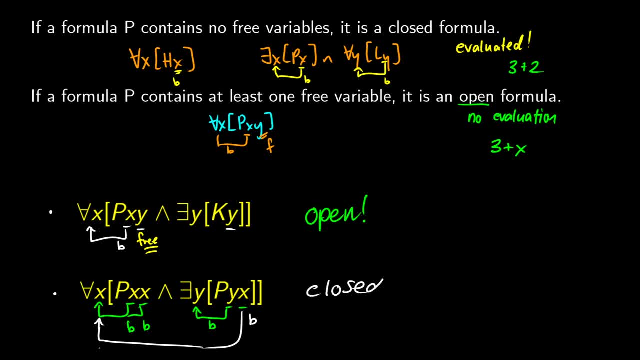 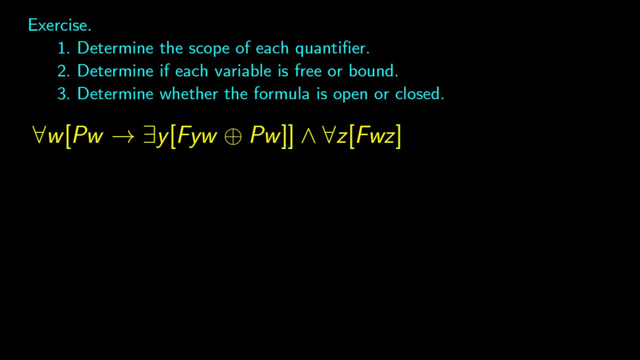 variables here are bound. we know this second formula is a closed formula. it can be evaluated. okay, that's everything I wanted to cover in this video in terms of content, so let's just do one final practice exercise with some operators that I didn't really use and more than two quantifiers. 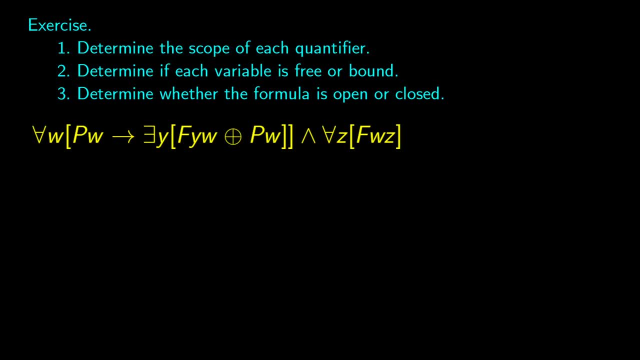 so, for this one, we're going to determine the scope of each quantifier, we're going to determine if each variable is free or bound, and we'll determine whether the formula is open or closed. and in order to do three, you have to do two. and if you have to do two, then you have to know one. 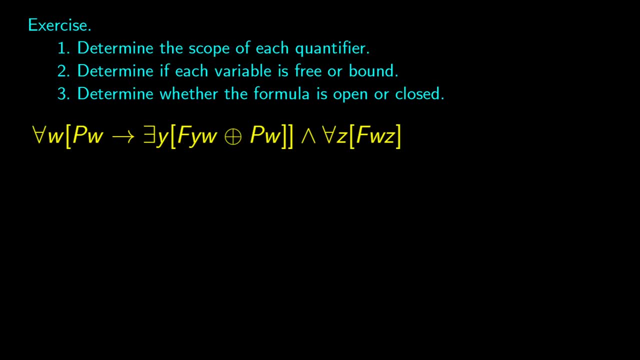 so it nicely builds on itself. so pause the video, beat me to it and here are the solutions for this. so we need to talk about the scope of for all w. we need to talk about the scope of existence of x out front. so we need to talk about the scope of x out front. so we need to. 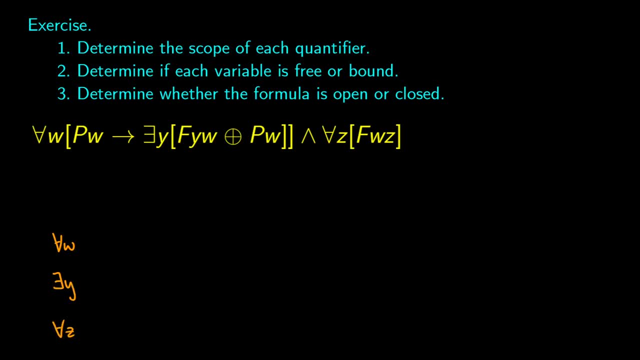 talk about the scope of for all z, so for all w, we're just going to follow the brackets. so for all w, we're going to have a scope of p? w arrow, exists a, y, f, y, w, exclusive, or p? w, and that one's not too. 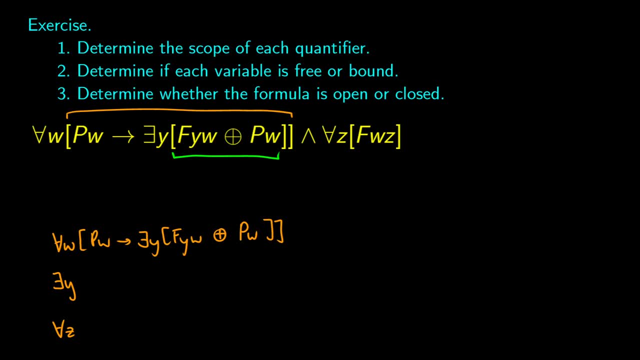 bad. we take a look at exists a y. we're just doing everything inside those brackets. so this will be f? y w, exclusive or pw. now notice that neither of those scope over the last one and for all z sort of lives in its own little realm here. so it's for all z f w, z and that would be the scope there. 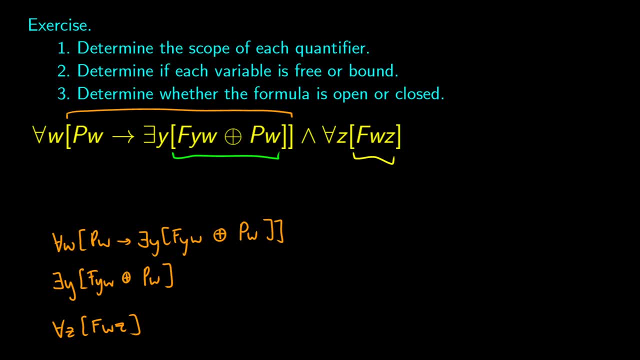 okay, so those are the scopes of each of our quantifiers. now let's think about the variables inside, and because we've determined the scope, figuring out whether each variable is free, or is free or bound is going to be rather straightforward for us. so we can ask ourselves: 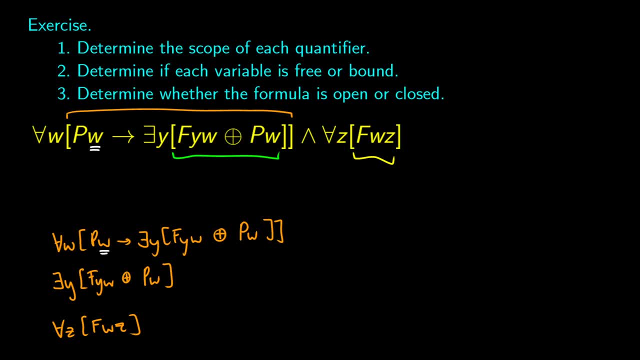 this w? well, this w is in the scope of for all w, so this is a bound variable. okay, i'm gonna get rid of these marks here. oh, i got rid of the whole question. that's not what i wanted to do. there we go. okay, exists a y, f, y, w, so what about this y? well, yeah, this y. if we take a look at our scope, 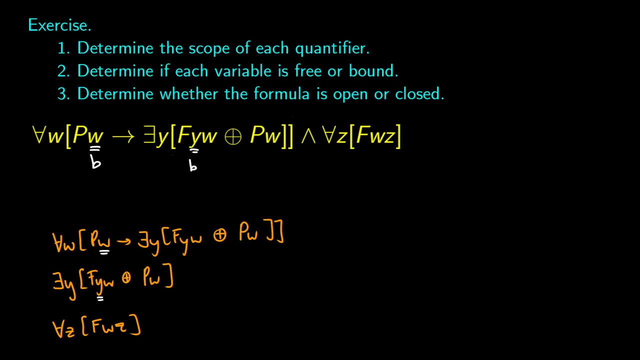 it's in the scope of exists a, y, so this one is bound as well. what about this w here? well, let's take a look at our w scope formula and we see, oh yeah, that w and f? y, w is in the scope of for all w. 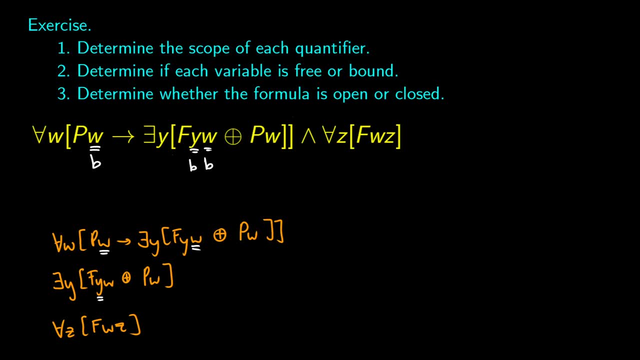 so this is also bound. what about p w? again, if we take a look at our all w scope, right there it is in the scope, so this is also bound. okay, we have two more left. we have f w z and that means we're looking at w and z here. so for this w and f w c, if it were to be in the scope,